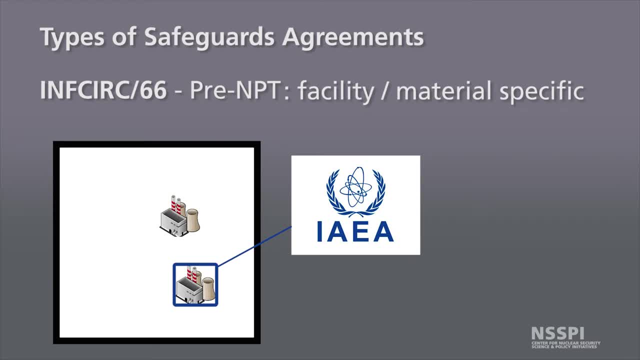 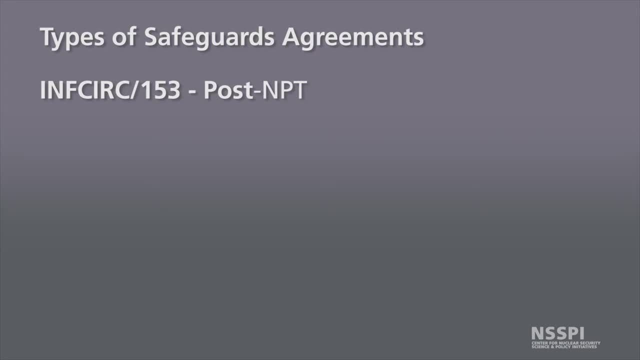 that occur at this one facility, not necessarily the other one. The next type of agreement is a nuclear instrument policy agreement, Which would be when the IAEA wants to use the GODG такой. This comes after the negotiation of the NPT and this includes Comprehensive Safeguards. 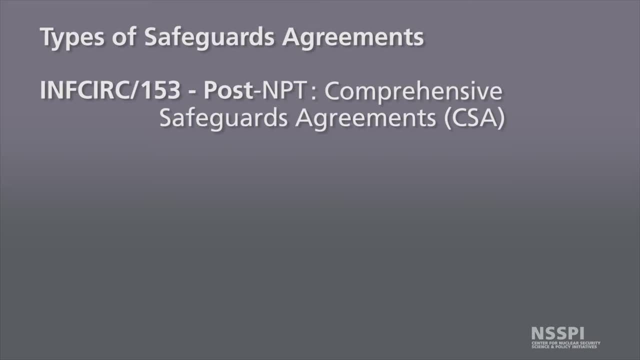 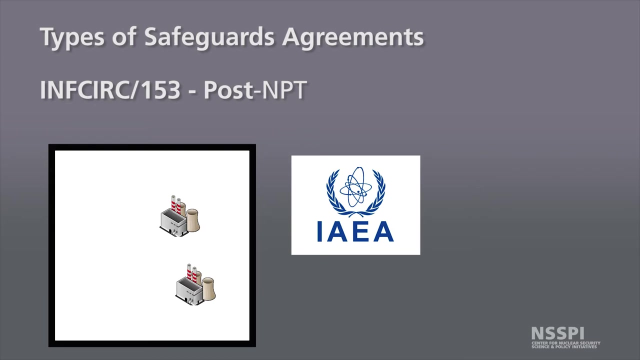 Agreements or CSAs, and those cover all facilities and materials within a non-nuclear weapon state party to the NPT. So if we look back at our fictional sovereign state here, if it has IMCIRC 153 Safeguards Agreements, then both these nuclear facilities are going to be included in the state's Safeguards. 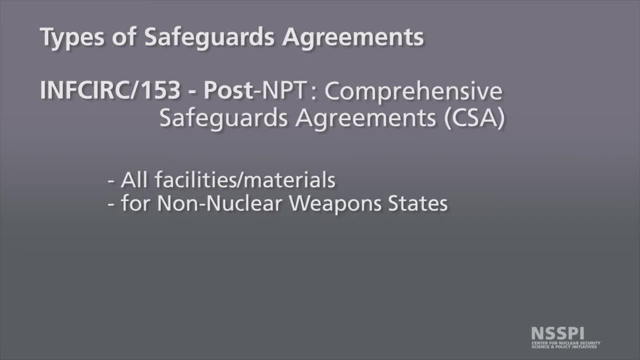 Agreements with the IAEA. IMCIRC 153 also includes Voluntary Offer Agreements and these are specific to nuclear weapon states. so those states that are codified as having nuclear weapons according to the NPT, They can conclude facility-specific Safeguards Agreements. 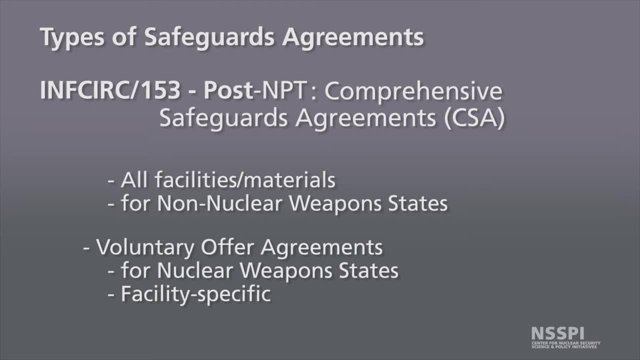 They are in the style of the CSA, Comprehensive Safeguards Agreements that non-nuclear weapon states have with the IAEA, but they are not to all the nuclear materials and nuclear facilities within the state. It's just the nuclear weapon state volunteers a specific facility with specific materials. 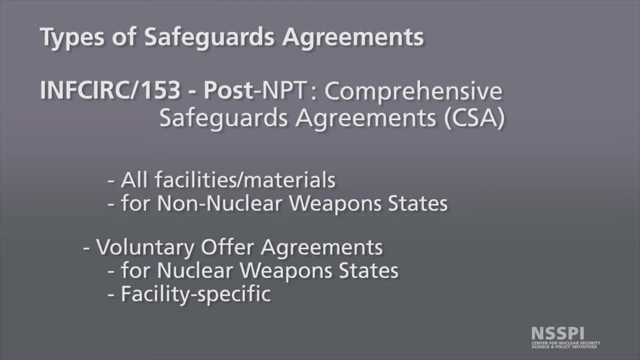 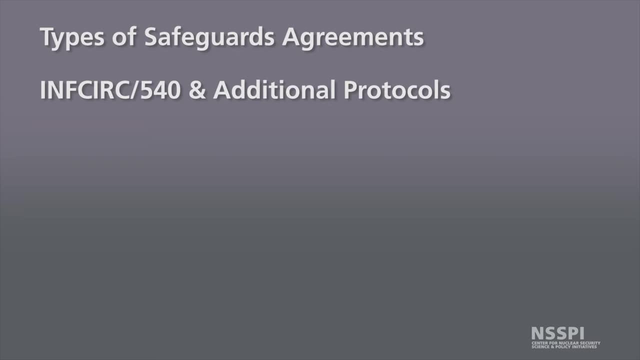 and gives the IAEA specific access that it negotiates. Then we also have the IMCIRC 540 and Additional Protocols and this is more directed at understanding and what the IAEA's going to want to do with the state. So this is the safe guard. it's going to be the safe guard of a particular nuclear facility. and it's going to rely on the IAEA. so that's the safe guard For the IAEA. it's going to apply to the IAEA and that's the IAEA. As for the UNDECLARED proliferation activity, the IMCIRC 153 and IMCIRC 666 Safeguards Agreements. 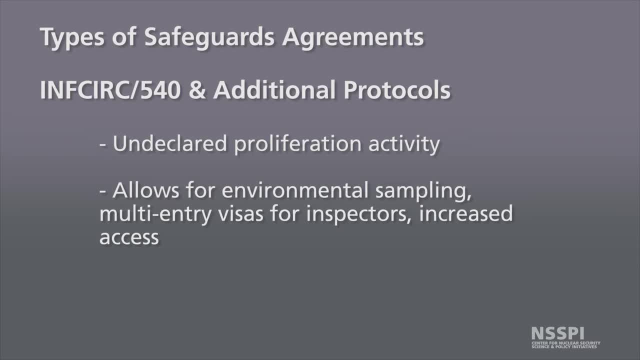 are applied to declared facilities with declared materials. IMCIRC 540 and the Additional Protocols gives the IAEA power to look at the rest of the state in general and allows for environmental sampling, multi-entry visas for inspectors and, overall, just increased access. 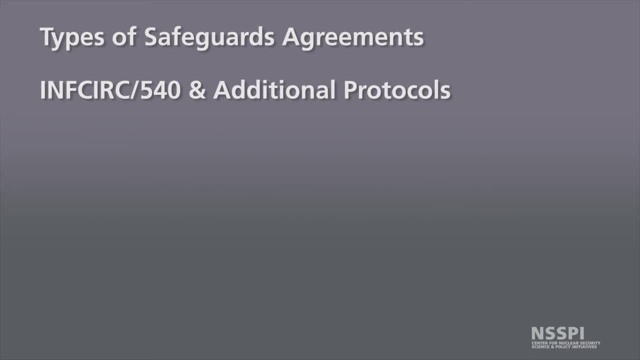 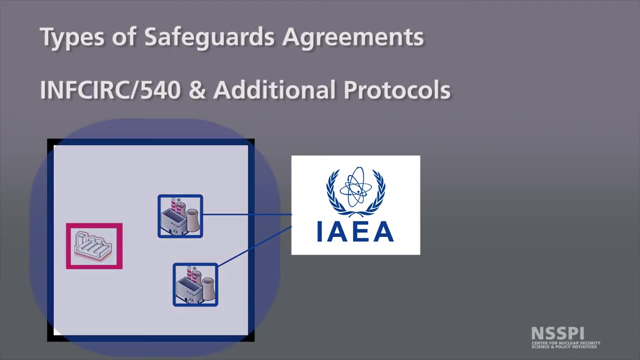 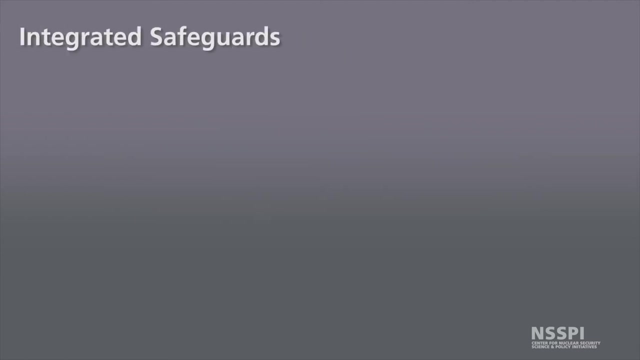 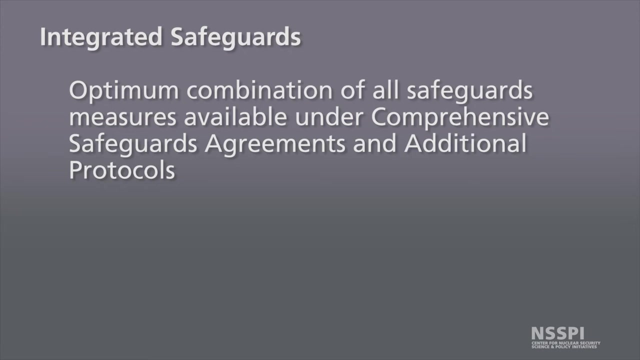 So if there is, say, some undeclared facility in our fictional state here, then the IAEA has some capability to detect this activity going on in the state as a whole. So another concept we want to discuss is integrated safeguards. Integrated safeguards is the optimum combination of all safeguards measures available under 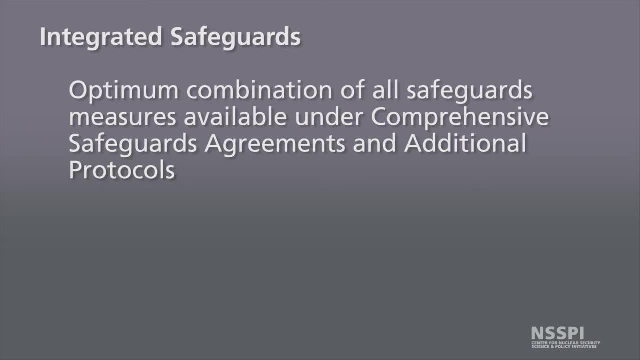 comprehensive safeguards agreements and additional protocols- And this is integrated. safeguards are applied to achieve maximum effectiveness and efficiency in the meeting of IAEA's safeguards obligations within the available resources. So the integrated safeguards concept is more efficient than kind of a maximal level of all safeguards at all times. 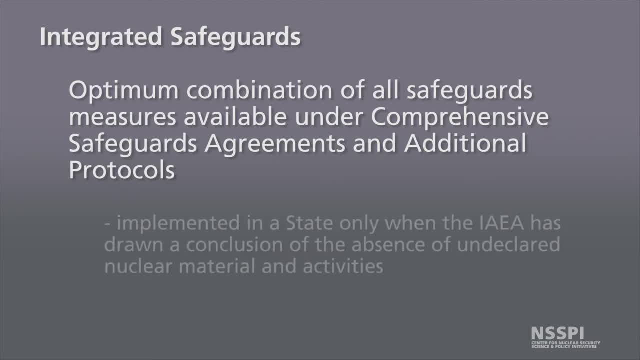 However, it is implemented in a specific way In the state only when the IAEA has drawn a conclusion of the absence of undeclared nuclear material and activities. So in the beginning the IAEA may take approach where it applies just maximal safeguards at 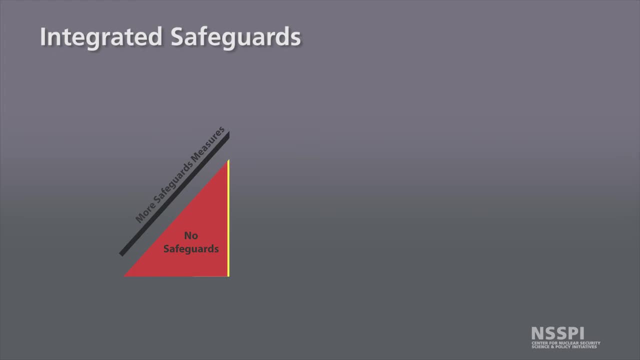 maximum levels. However, once the absence of undeclared nuclear materials and activities can be verified and can be concluded, then it may be possible to shift to more of an integrated safeguards approach which optimizes And streamlines things for effectiveness and efficiency. Under integrated safeguards, measures may be applied at reduced levels at certain facilities. 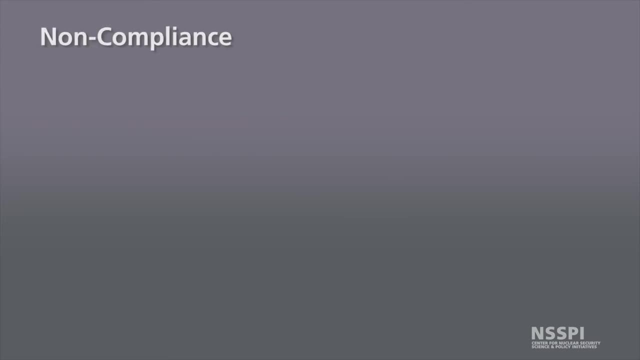 in some cases. Another concept that needs to be discussed is non-compliance, And this refers to a violation by state of its safeguards agreements with the IAEA. So some examples of issues of non-compliance are the diversion of nuclear materials from declared nuclear activities. if this occurs, then a state may be found in non-compliance. 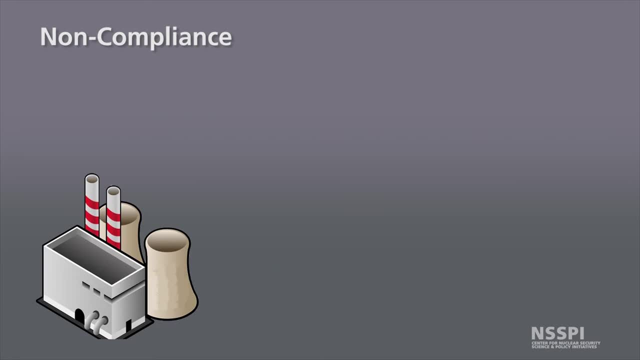 with its safeguards agreements. Another example could be failure to declare nuclear material required to be placed under safeguards. If additional nuclear material is found that was never declared, then the IAEA may find the state in non-compliance. If a state has an additional protocol, the failure to declare nuclear material is not. 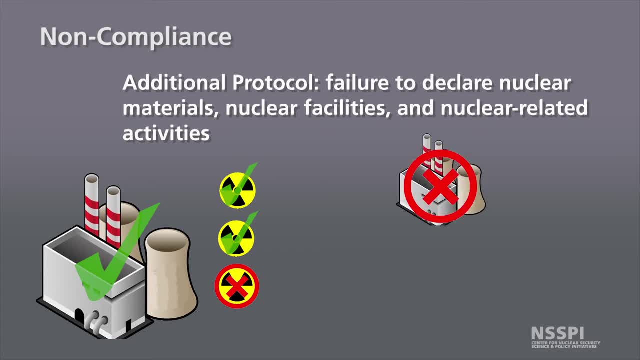 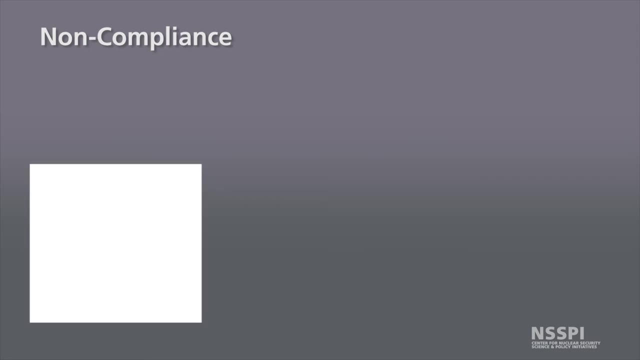 declared. If a state does not declare nuclear material, nuclear activities or nuclear related activities would be a cause for non-compliance. Violation of agreed recording and reporting system. any obstruction of the activities of IAEA inspectors could be a cause for non-compliance. conclusion or interference with the operation. 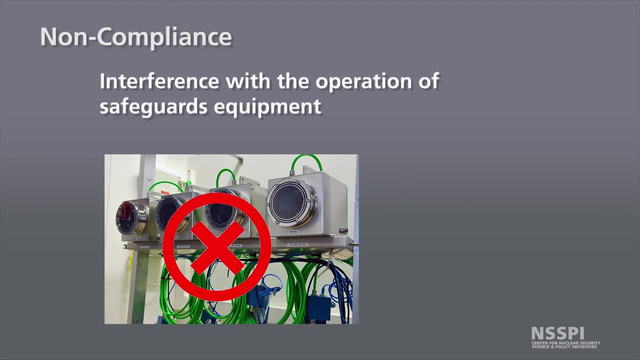 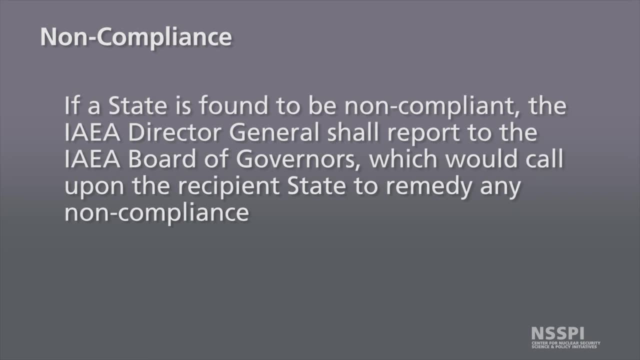 of safeguards. If a state is found in non-compliance, the IAEA Director General shall report the non-compliance to the IAEA Board of Governors, which would then call upon the recipient state to remedy any non-compliance that has been found. 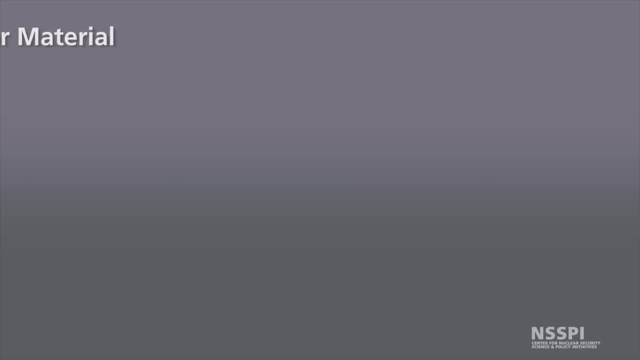 There are two general types of non-compliance, the first being the diversion of nuclear material in non-compliance for schools and drawing upon the levels of compliance and protection kind of requirements. orемуplease behold, your materials are not technically required in adult equipment to be yogurtable prototypes. 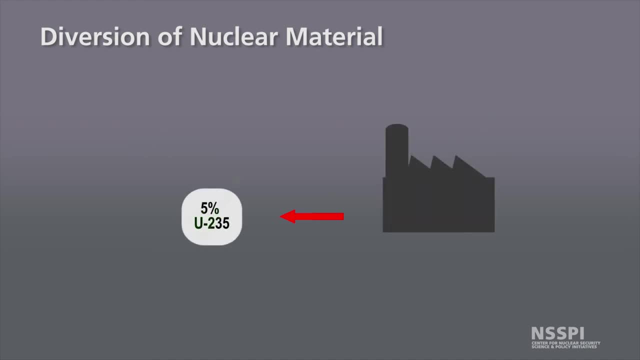 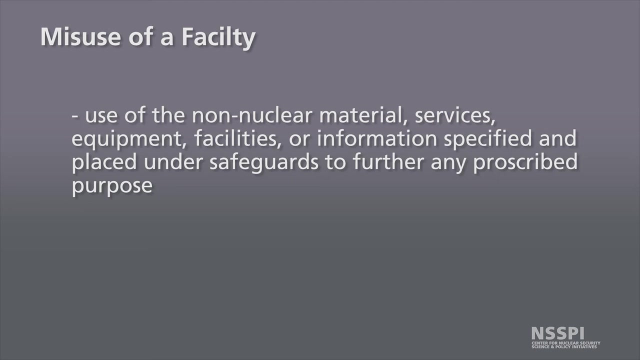 O feel good about your water and probably watch system measures against you. at what level you do not get TaxBob's Mr forbread and worth it. Everyone is definitely podcasting today. Somebody has just written a comment, they have just uploaded their post and they have. 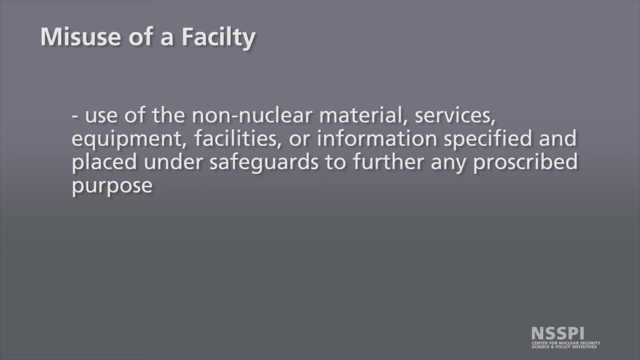 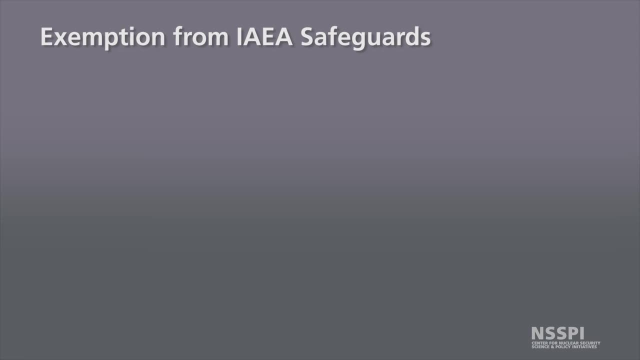 流ed the line from bottom-up. Does this make sense? I think so, Okay. or proliferation activity. There can also be cases of exemption from IAEA safeguards. A state may request exemption of nuclear material up to certain specified limits If the state 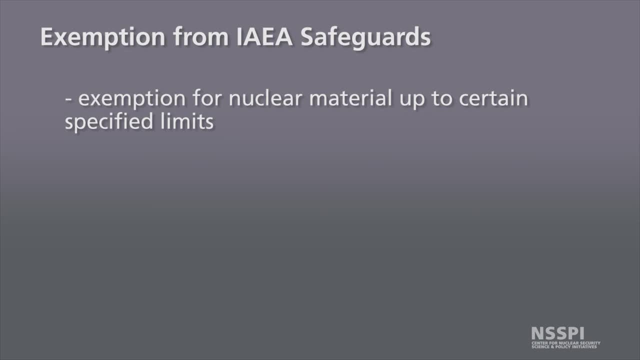 has a very low amount of nuclear material within it, then it may request and be approved for exemption from nuclear safeguards. A state may also request exemption for specific nuclear material that is related to a specific intended use. This could be gram quantities that are used as a sensing component within nuclear detection equipment and instruments, Or it